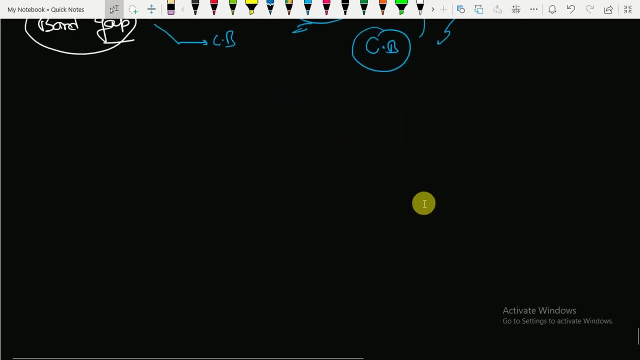 like to explain or differentiate conductor, semiconductor and insulator as per their band theory. so let me draw a chart that is for conductor or semiconductor and for insulators. now, in case of conductors, energy band, energy band overlaps. in case of semiconductor, energy band or energy gap, you can say EG is less. 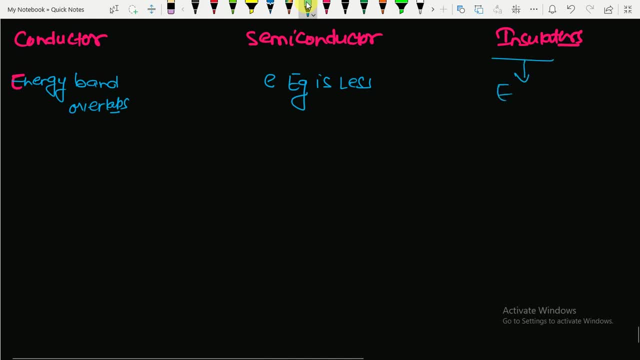 and in case of insulator EG, that is, energy gap- is very more so that electron from conductors valence conduction band will not jump to valence band so that there will be no conduction. now you can say that in case of conductors as energy band or energy gap. 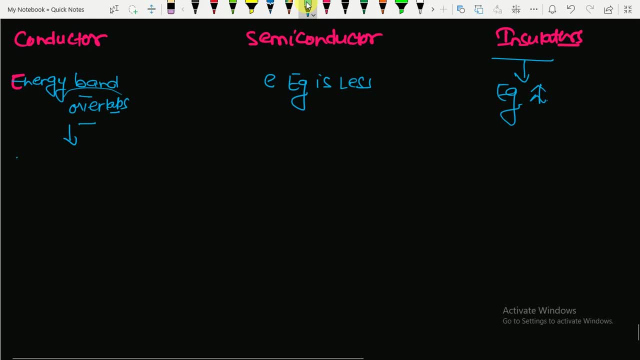 is overlapping. you can say that there, if there will be slight excitation that will cause electron to jump from valence band to conduction band, and that is, with slight excitation, slight, slight excitation, electron will jump from valence band to conduction band. okay, now in case of 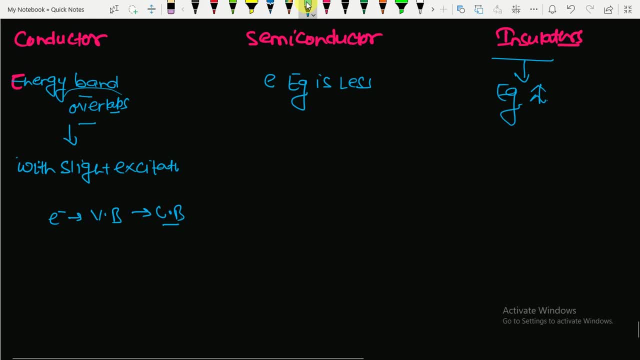 semiconductor as it the easy is less, that is, band gap is small, so it requires some small amount of energy. either you can provide it in form of thermal or you can provide it in terms of photon or equals to h? nu. it will require a small amount of energy to pass into the conduction band. that 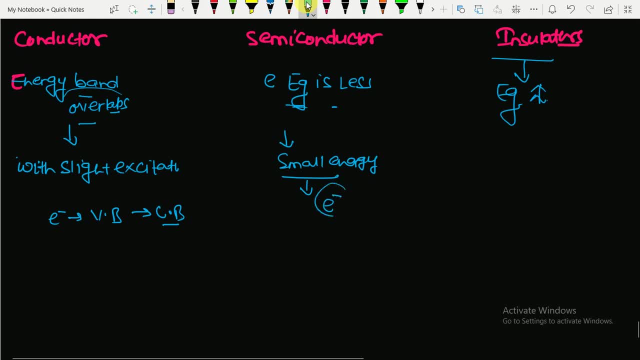 is the electron which is placed in a valence band will require a small amount of energy to just jump from valence band to conduction band and hence conduction will possible in case of semiconductor, because easy is less, that is, air gap is less. sorry, sorry, air gap i am talking about. 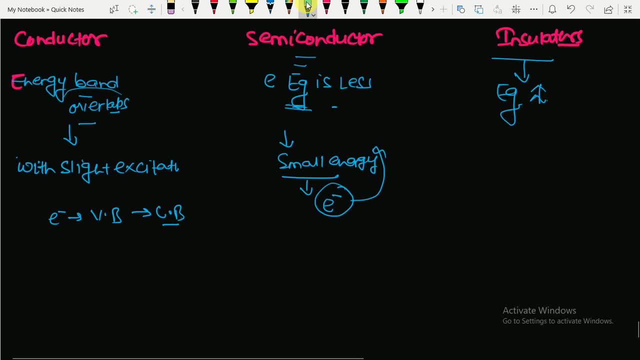 energy gap- now you can say that in case of semiconductor easy- varies from near about 0.12 electron volt to 5.3 electron volt. now, in case of insulator, as electron do not leave the valence, valence band, even by thermal excitation, why, why? why, in case of insulator, if you provide the thermal excitation to that insulator, 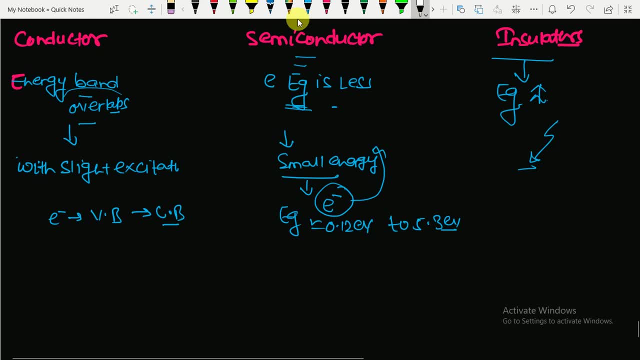 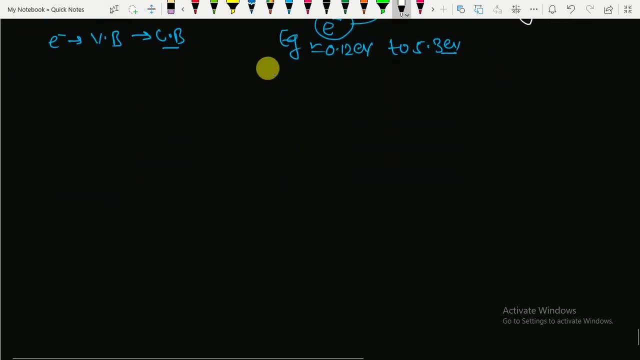 there will be. there will be no electron jumping from valence band to conduction band because their energy gap, that is easy, is very high. that is, you can say that it's nearly 6 electron volt. electron volt energy. now let me show you How does possible? now, in case of conductor, you can say that: 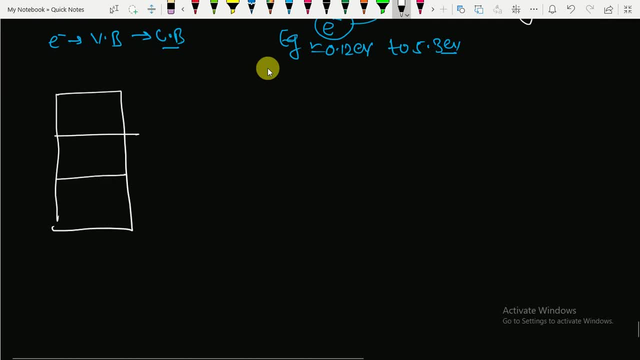 there will be overlapping of valence band and conduction band. so this is conduction armlet, say, and this is valence band, and they're overlapping. I presented by you can see this is the overlapping easy that is the band Fernand – energy gap will bring equals to 0 electron boat. 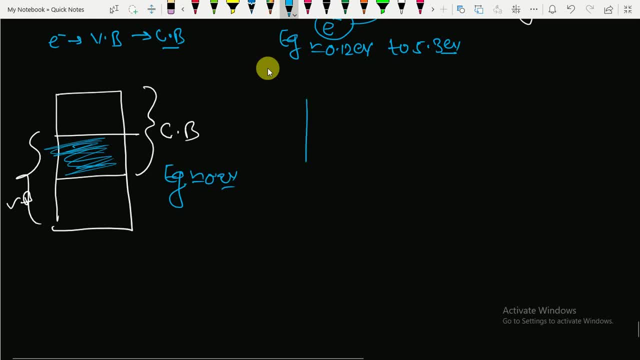 but now, in case of semiconductor, energy gap is very less. so you can say that there will be a transmission of electron from valence band to conduction band. if you provide little amount of energy, that is nearly equal- equals to one electron volt- to the electron now in key. this is conduction band and this is valence band. 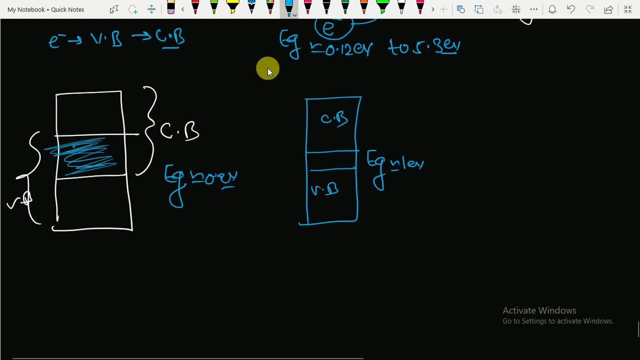 if you will, in conduction band and valence band there will. there are holes on in conduction band there are electrons. so if you, if we will provide the energy near about one electron volt, the electron will start jumping from leaving the valence electron valence band and occupying the position of 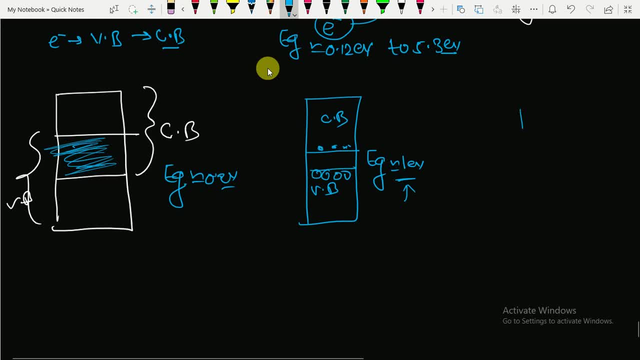 conduction band. now, in case of insulator, you can say that the energy gap is very much, very high. that is nearly equals to easy, nearly equals to six electron volt, which is very high. so then there will be no conduction. in case of insulator, solid atoms very close to. 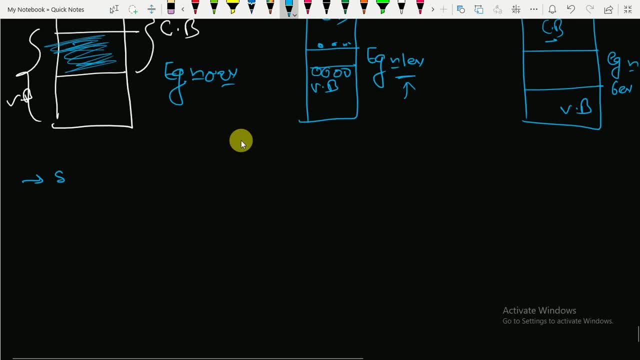 each other. let me discuss you some point. in case of solid, atoms are very close to each other, electrons experiencing attractive force from other nucleus also. so you can say that in case of solid, if you will talk about the electronic configuration, electronic force of attraction or repulsion, you can say that: 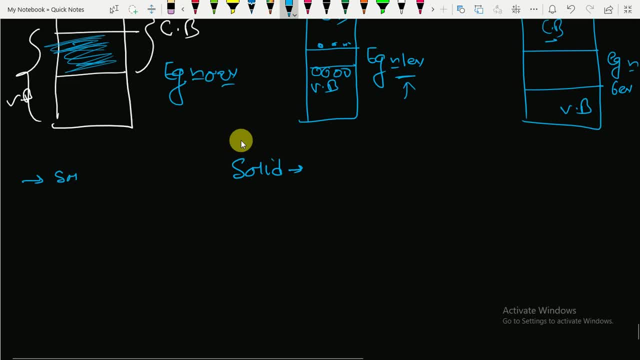 in case of solid atoms, are very close to each other, that is, atoms very close to each other, electrons experiencing attractive force from other nickel nucleus also. that is, the electrons are in periphery of other nucleus also, so they are experiencing some of the attracting force, so that energy will. 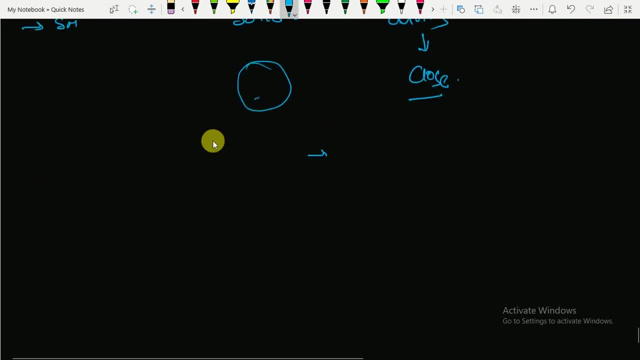 vary energy and that that variation energy will really will call energy band. now fully filled band, electron do not participate in conduction. if the energy band is fully filled, if the energy band is fully filled, then there is no need to electron to, there is no need of electron to take part in conduction. now let me 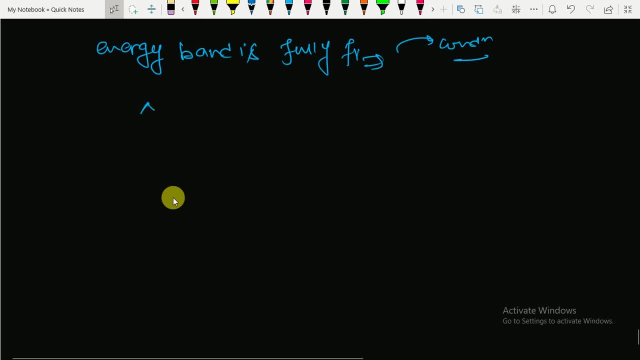 show you what is easy that is. energy band will throw energy chart. now this is energy level. that is, let's assume, conduction band and this is valence band, valence band. this is conduction band. I am plotting this curve against energy, energy plot, conduction band and this is valence band. and this gap, that is the gap of energy. 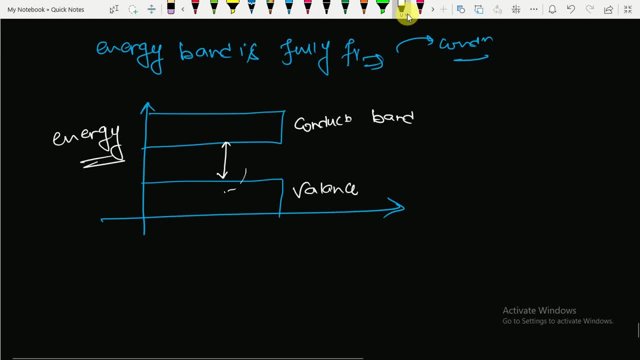 required to electron to jump from valence band to conduction band is E G, that is the band gap. now this is known as E C and this loop is valence band and the leg work or range will be than called E C. collect score is nothing. A har censored. 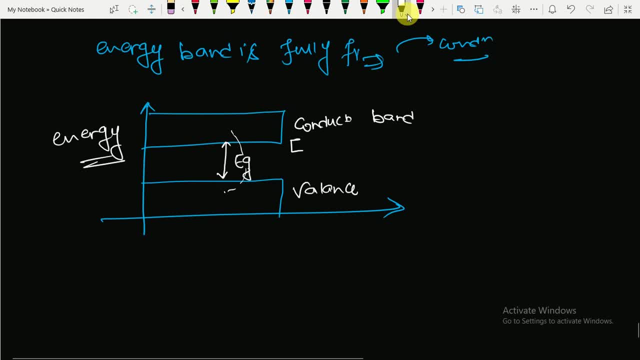 volume of verse, river heavy. more interesting nature of Kepler graphs. if you look, don't worry. if it's hard tojà, take a look. if it is is easy capability, so just just. And this is EV. What is EC and EV? I will explain. EV is the lowest energy level of conduction band. 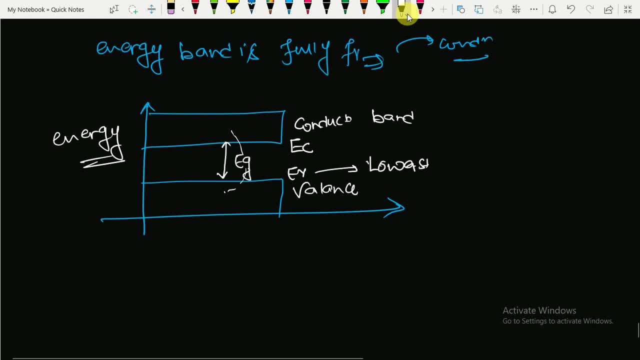 Lowest, That is, EV is the EC is the lowest energy. Now this electron will jump from valence band to conduction band And this energy is known as energy gap. Now EC is known as highest energy level of lowest energy level of conduction band, EV is known as highest energy level of valence band. 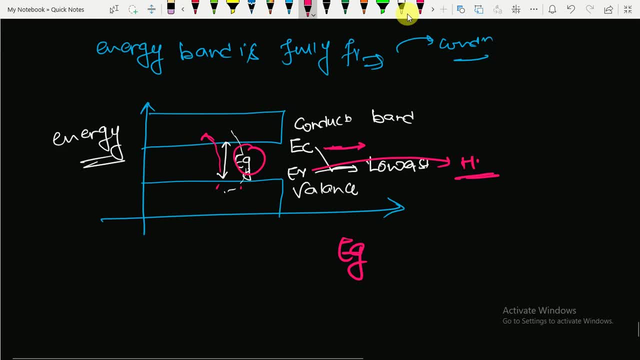 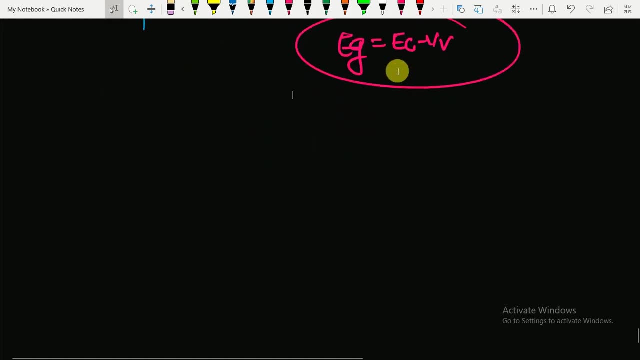 Now EG is energy band gap or forbidden energy gap. Forbidden means why? Because in this reason there will be no electron. So it is known as forbidden energy gap. And EG equals to EC minus EV. This relation is important. Now, valence electron in conduction band do not participate in conduction. 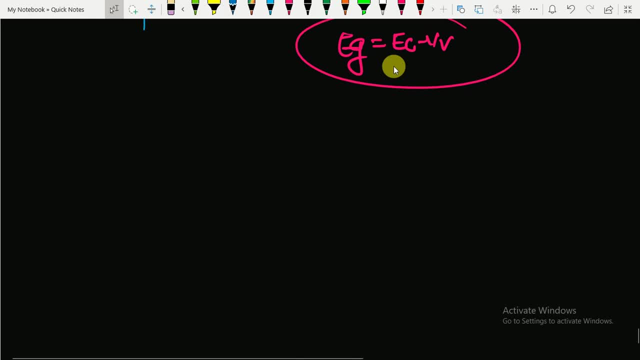 Do not accept the applied voltage. That is, if electron will jump from valence band to conduction band, then after the electron raise to the conduction band, there will be no, the electron will not participate in conduction and it will not accept the applied voltage. 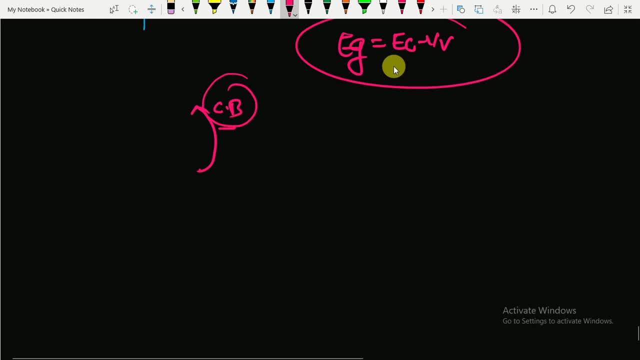 That is, either you will apply any energy source or to any voltage to that electron. It will not accept any sources. to just conduct Now let us assume EG is the lowest energy level of conduction band, So EG is known as highest energy level of conduction band. Let us assume EG is the lowest energy level of conduction band, So EG is known as highest energy level of conduction band. Let us assume EG is the lowest energy level of conduction band, So EG is known as highest energy level of conduction band. 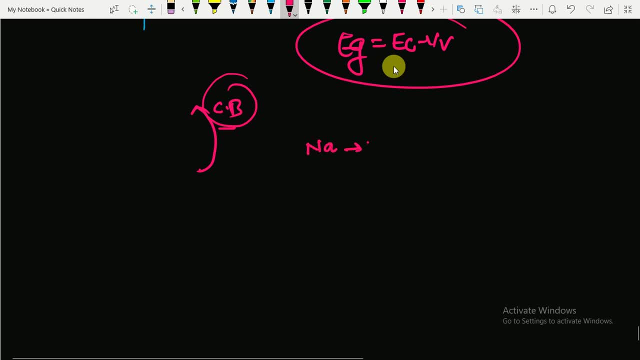 Let I am taking sodium atom. It has 11 electron, that is, 1s2, 2s2, 2p6, 3s1, 3p0.. This is the valence electron valence band and this will known as conduction band. 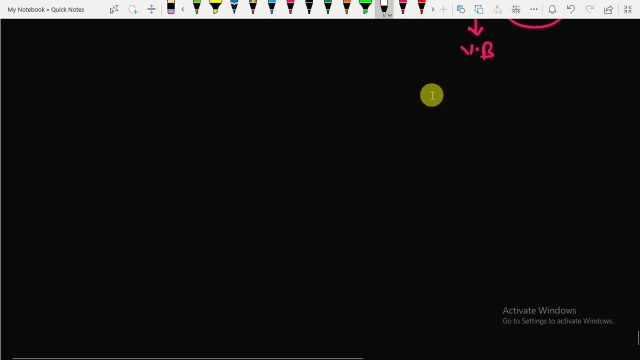 Conduction band Now in forbidden gap. in case of forbidden gap, why there is? there will be no electron. because to conserve momentum, that is, for the conservation of momentum, that is, MBR equals to NH by 2 pi- electron can only present in band. why electron can only present in band? UPSC can ask a. 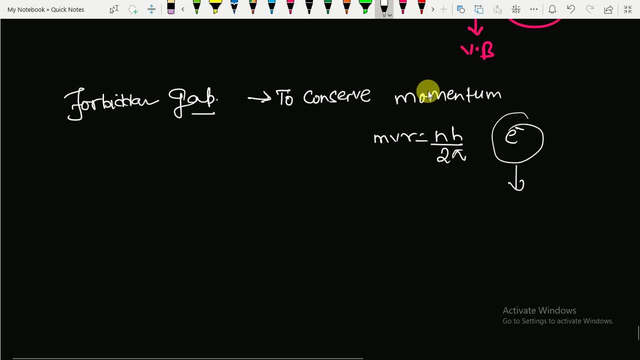 question: why electron? we can only expect in electrons in bands. so you can say that to conserve momentum, that is to follow the law of conservation of momentum, that is, MBR equals to NH by 2 pi. electron will only present in the bands. now, in case of metals, in metals, the electrons of electron cloud. 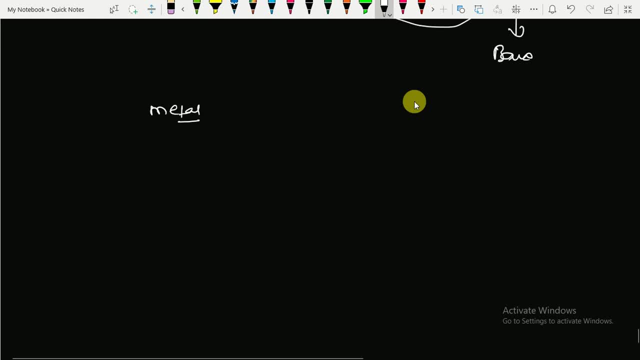 participate in bonding and also they are free to move, therefore participate in conduction. in case of metals, I have already told you, there are pool of electrons, so they will participate in conduction. now let me give you a relation. EG, that is energy gap for energy, band gap at temperature T, equals: 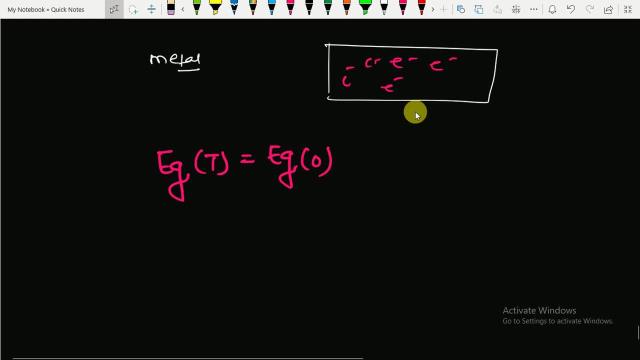 to EG at temperature 0 Kelvin minus beta T. this is the important relation you have to remember. what do you mean by term as energy T narrow value? what do you mean by termة is very important. you already understood what energy GAP is. energy GAP is' the material at T Kelvin and its 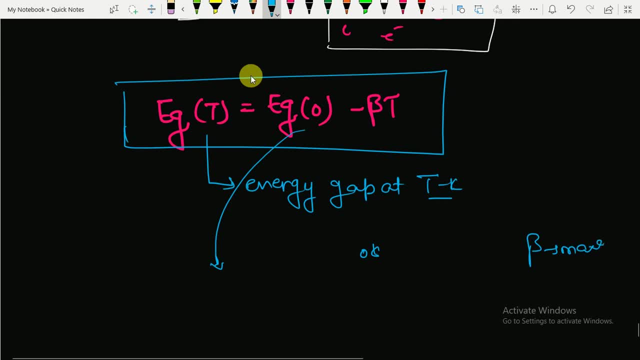 depth of T is the sorry. so the distribution is ättä'f't, that is energy Wi, E, g, my fu, e of T. that is energy gap at T Kelvin. that is energy gap at Q Kelvin. that is energy gap at T kelvin. and EG zero energy gap at zero Kelvin. beta is the material constant, material constant. now, this relation is very much important. you have to remember it now. 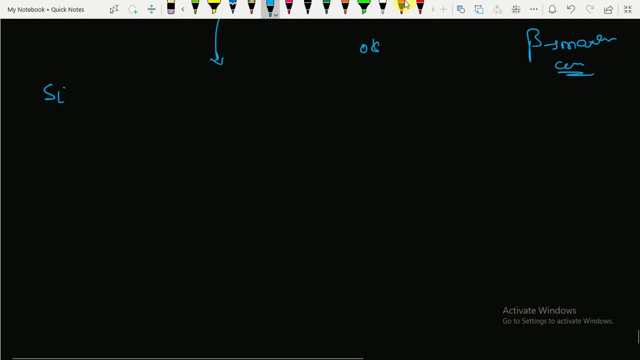 I would like to give you some practical data for silicon and follows the relations germanium. silicon and german germanium are the heroes of semiconductor, as we already know. at 0 kelvin from that relation, ez0 will be 1.21 electron volt and at 300 kelvin 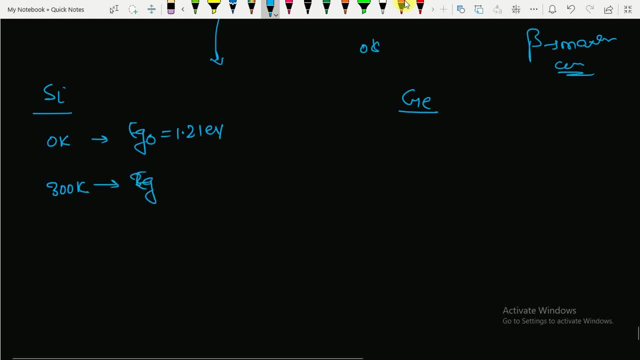 ez0, ez300 will be that ez300 kelvin will be 1.1 electron volt. for germanium, at 0 kelvin, ez0 will be 0.78 electron volt and at 300 kelvin it will be 0.7 electron volt. 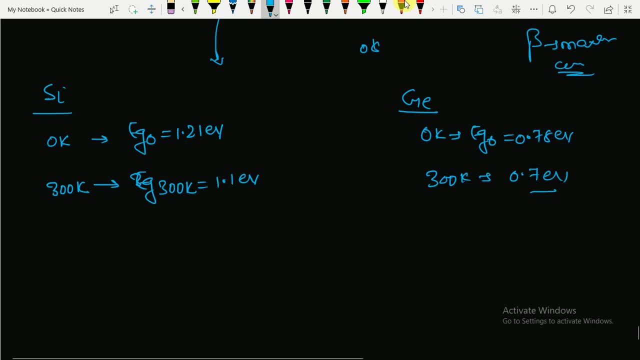 now let's talk about insulator. insulator- let's know the very much interesting point about insulator, that is, when an insulator in molten state, when an insulator in molten state it is a good conductor. now semiconductor at 0 kelvin will behave like a insulator. 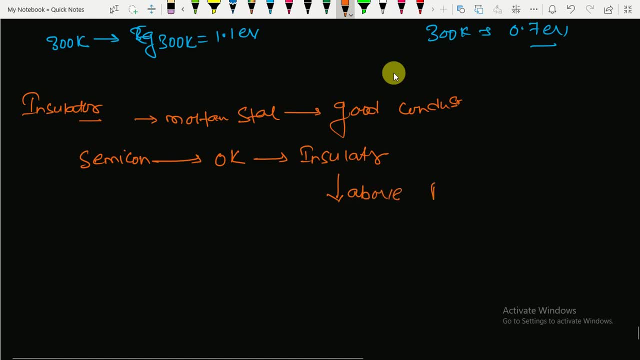 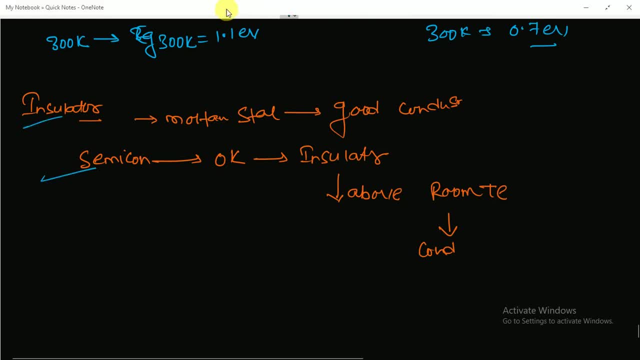 points in a sarsen reason question. example of semiconductor is germanium silicon gallium arsenide, Because我們 clear mix cadmium andARK. gallium arsenide is used in remote led silicon germanium. we all know very well. gallium arsenide, which is used in remote led silicon germanium, we all know very well. 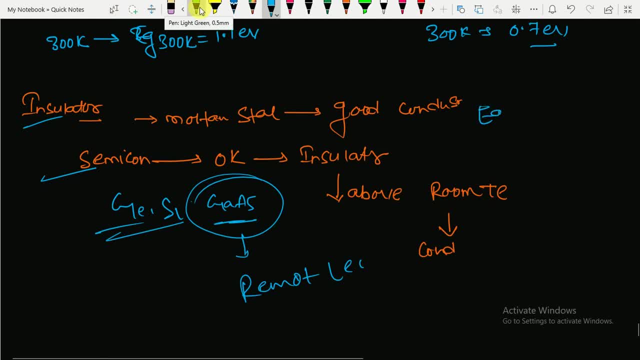 Now ego is equals to HCO2, as in drinking water. now E G is equals to HC 4 G. so what is this arrival point that we'll know in fast forward? 내 hc by lambda. This is a relation of energy gap or energy. You can say that. 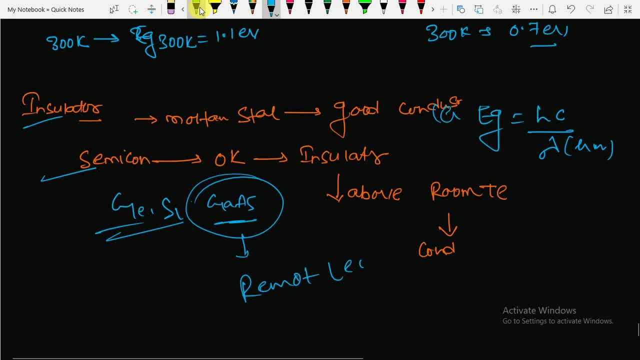 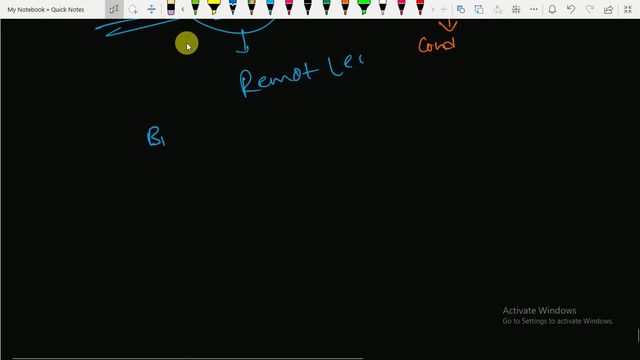 lambda is in micrometer, Hence EG will be in electron volt. Now how an insulator breaks, that is breakdown mechanism of an insulator. So there are three ways, That is, it can be a thermal breakdown, It can be an electric breakdown or it can be a chemical breakdown. 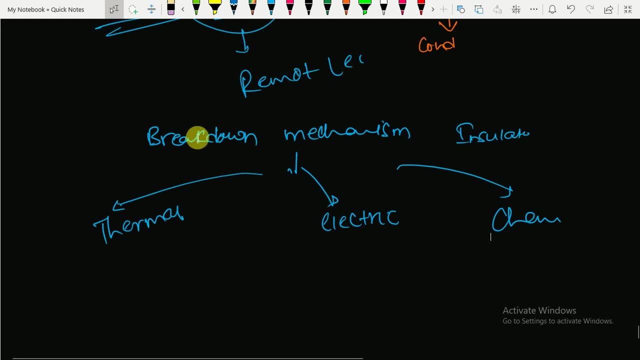 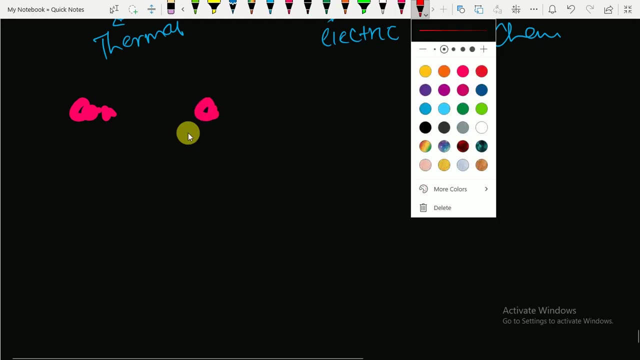 We do not need to go in very much detail, and if I have to clear it then I will go in my next next few slides. Now start. I am going to start conductor, Sorry. So Hume's law law and electrical conductivity. 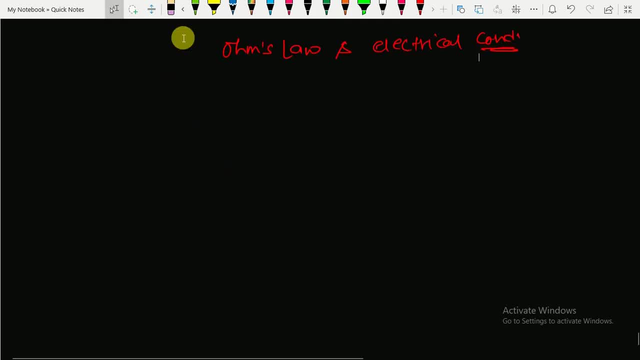 In case of conductor. we all have read this topic, but I would like to explain it. If you want to go in deep, you can refer videos of analog electronic in my playlist. I have completed in very depth, So let us take a conductor. 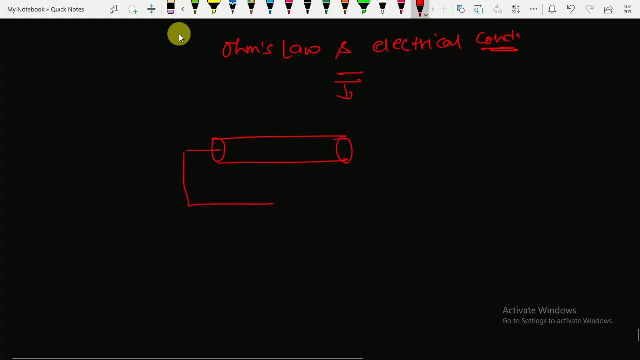 And I have connected it with a battery. Now I have connected with a battery V or E- You can say that V or E And I is the current flowing through that conductor- And these are the electrons which are starting to started to move from positive terminal to negative terminal. 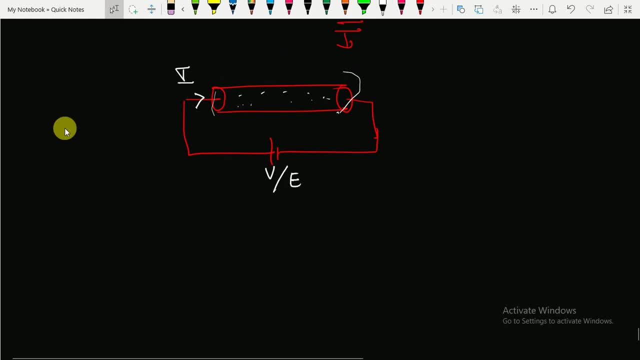 Now let us take some assumption or some notations. That is N, is the free electrons, That is per meter cube, That is electron concentration or charge carrier concentration. I have explained it in very much detail. You can refer my analog basics lecture. 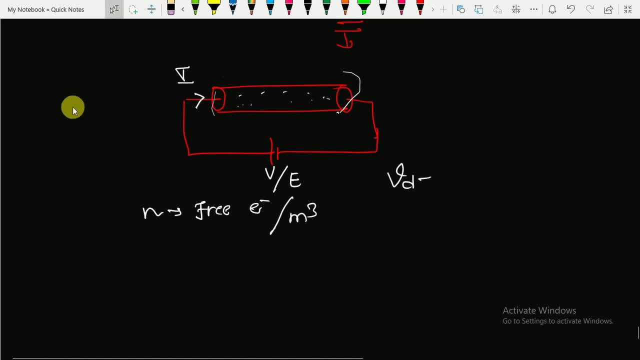 Now I am taking as Vd is as drift velocity. Now, what do you mean by the term drift velocity? It is the average velocity acquired by the electron under the influence of electric field. is drift velocity, That is, electron will observe or electron will face some impact? 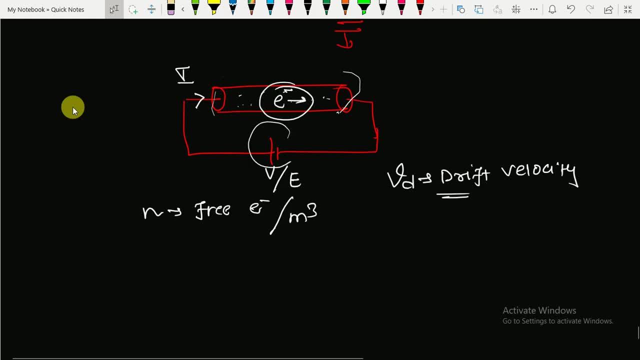 That is, electron will observe or electron will face some impact. That is, electron will observe or electron will have effect. onrak ettity: Randomness of Electron. Randomness is inversely personal to drift velocity. Please remember this topic, This point. 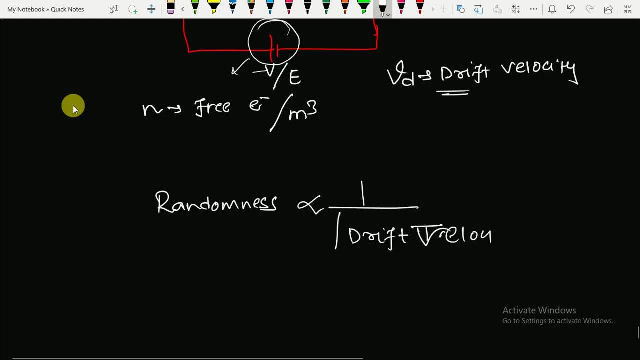 drift velocity. as drifting increases, randomness decreases, so you need to remember this because they can ask, or they have asked, question related to this. now let me introduce a new term, tau, which is known as average collision time. i need not to go in depth with this topic, in case 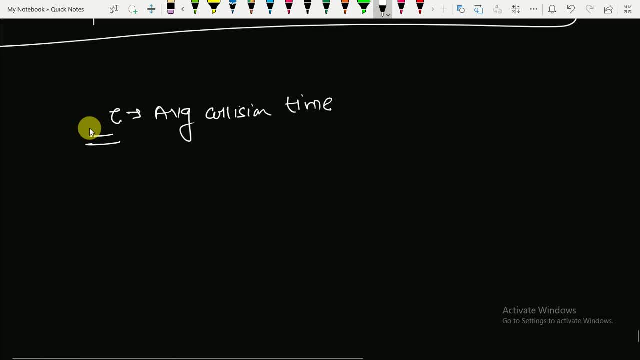 of material science, engineering. if i will go through the technical portion, that is for electrical and magnetic material, i will explain you in very much detail or you can refer my analog electronics lecture now. the average collision time, tau, will be inversely proportional to root of temperature- this term you have to remember- as temperature will increase collision. 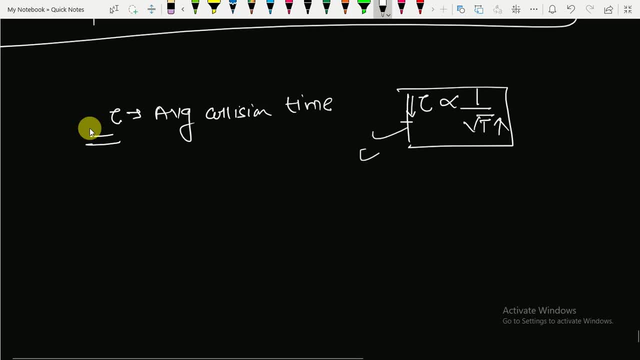 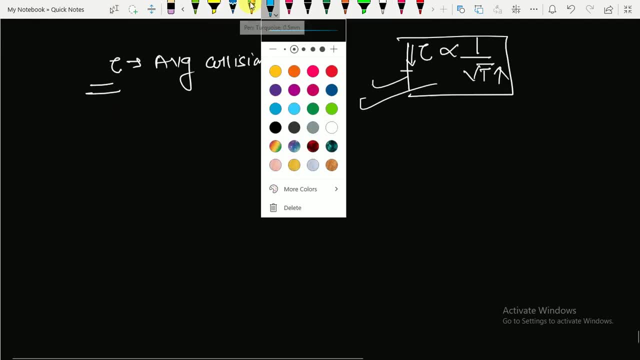 will decrease. kindly remember, in earning services, damnation. you can expect question related to this now. now, as per ohm's law. you can expect question related to this now, as per ohm's law, as we know that v is directly proportional to i, for removing proportionality constant v equals to r into i. 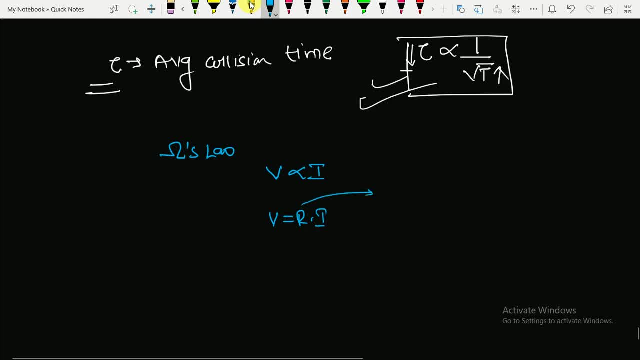 but remember: r is not the function of applied voltage and current. always remember r is not the. please remember this, this point: r is not the function of voltage and current. now, as we know that r equals to ρ into l by a. if i am taking a conductor of size of like this, having cross-sectional adia, a and 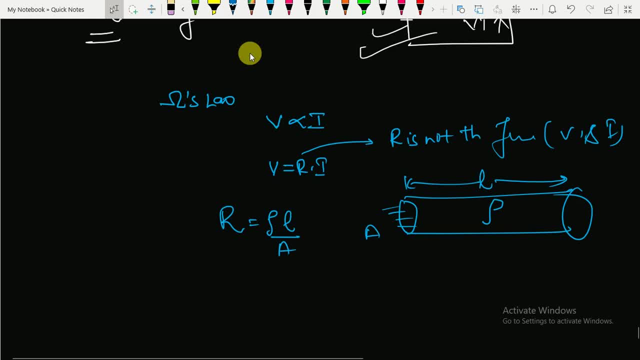 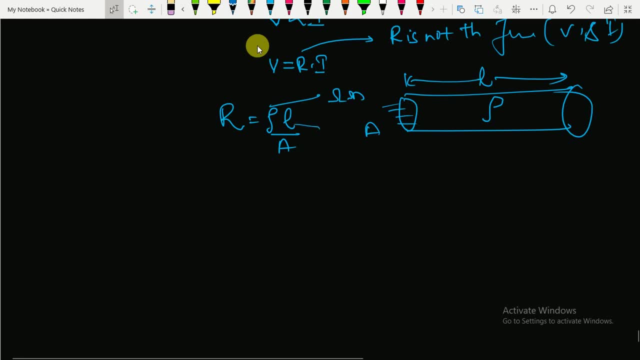 its length is l, so you can, and its resistivity is ro. you can say that r equals to rho into l by a rho. e is the resistivity of the material that is in oh interior is the length of that conductor. s is the cross-sectional adia of that semiconductor sigma equals to one by rho. sigma is: known as conductivity, so as rho equals to rho, unit of rho equals to t. so if we look at the data, this is corresponding to the conductors. and on allwork of the semiconductor there is aี้ is called as 태 chin computer, and this number is very easily included, however, so youtube can write it and we need to add this number. 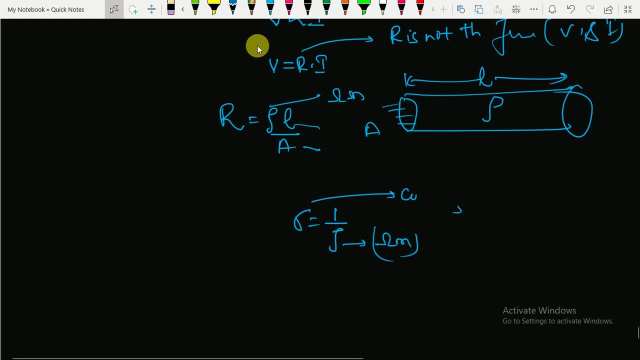 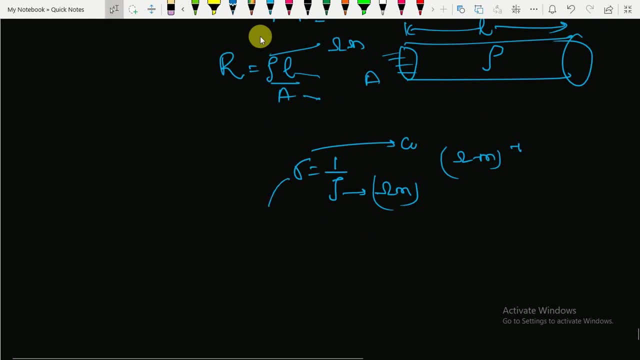 is ohm meter, so electrical conductivity unit is ohm meter, inverse per ohm per meter. you can say: what do you mean by the term sigma? sigma will represent the current carrier capability of that material, that is, the material will carry how much amount or, without any obstruction, how much amount. 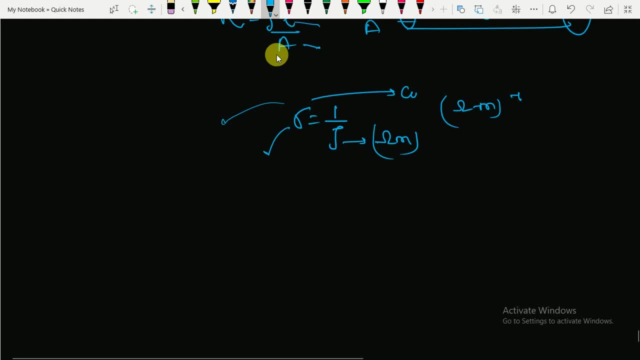 of current it will carry. that is the current carrier capability, current carrying capability of that material. so you, you, you should know the fact that resistance is not the function of applied voltage and current. so you can say that v equals to r into i and using r equals to rho into. 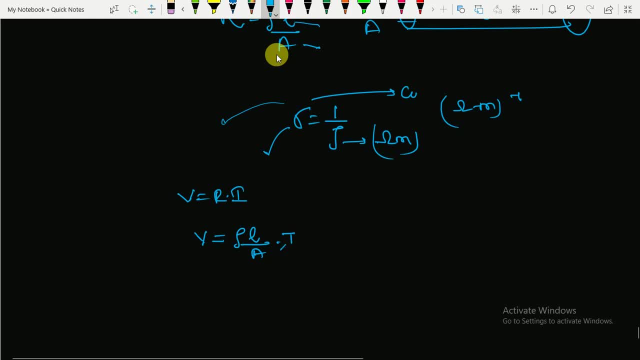 l by a, l by a into i. now, transferring this i- now you can write it as i by a equals to 1 by rho- into v by l. through this equation you can say that: and as we know that current crossing per unit area, that is, i by a, you can say that the current density, j, that is its unit, is ampere. 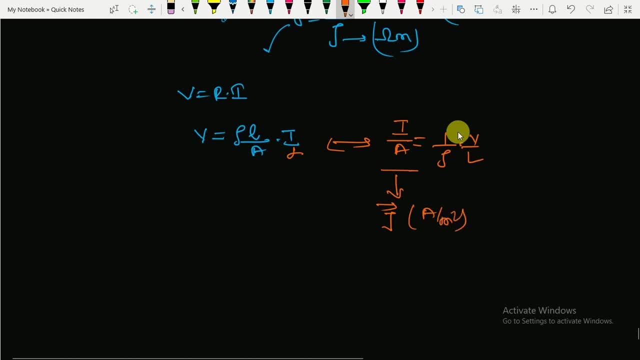 per meter square. now you can say that this is j equals to 1. by rho is sigma potential per unit length. voltage drop per unit length. is electric field e. so you can say that j equals to sigma. this is the another form of ohm's law. you need to remember this point anyhow, is it's the another?